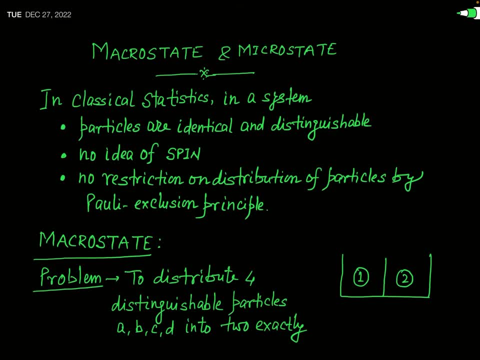 In today's lecture we will discuss macrostate and microstate. Actually, the concept of macrostate and microstate is very important in the study of statistical mechanics. Whenever you will study the classical statistics or quantum statistics, always we need the idea of macrostate and microstate. So 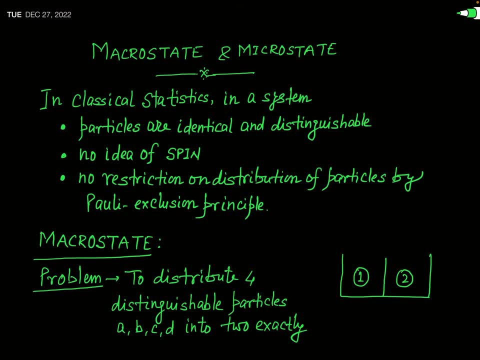 today's lecture is very important. This is a very important fundamental fact And after knowing this concept, the study of statistical physics will be very easy to you. So be serious, watch the video seriously And I hope, after watching this video, your concept about the macrostate and microstate will be very 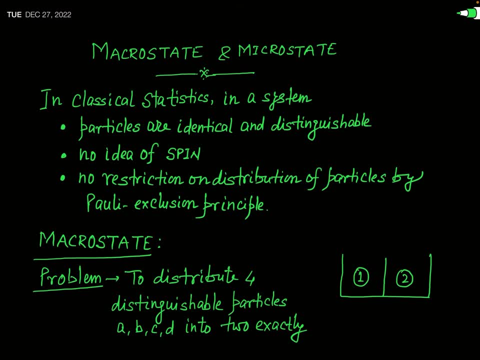 clear. Actually, I am going to explain the macrostate and microstate by a simple example. As you know, this idea of macrostate and microstate is needed for the study of both classical statistics and quantum statistics, And I hope, after watching this video, your concept about the macrostate and 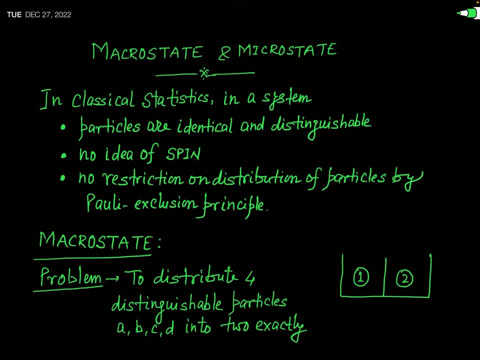 quantum statistics will be very clear. Actually, I am going to explain the macrostate and microstate, But in this lecture it is limited to explain the concept of macrostate and microstate only for classical statistics. When we will talk about the quantum statistics in the forthcoming lecture, then we will. 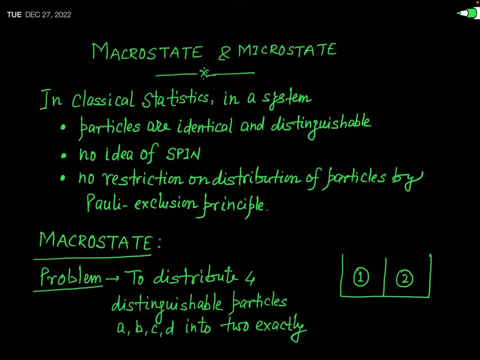 again see this concept. This concept will be actually then extended to quantum mechanical systems, but in the present lecture. So we are just limited to our discussion for the classical statistics. When you talk about the classical statistics for a system, you know that a system is actually. 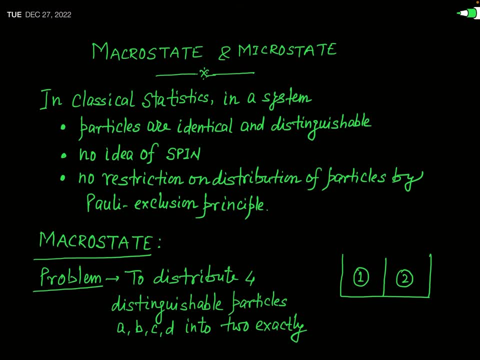 composed of a large number of particles that may be atoms, molecules or any other particle, And in classical statistics we simply consider that the particles of the system are identical but distinctly visible. It means when we study the classical system we assume that our particles of the system 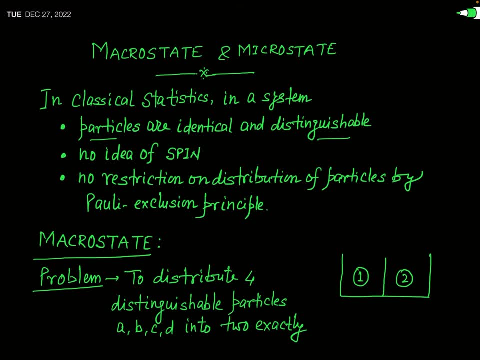 may be this- are actually distinct And that's why we can label that particle. We can name the particle like A, B, C, D And so on. Okay, As you know that the spin is purely a quantum mechanical property of particle, 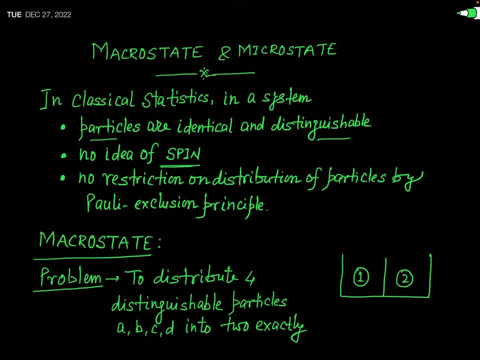 So when we talk about the classical statistics, we never think about the spin of particle, because this spin of particle plays a very important role in distribution of the particle in different quantum states. And in case of classical statistics, as we do not take into account the idea of a spin, 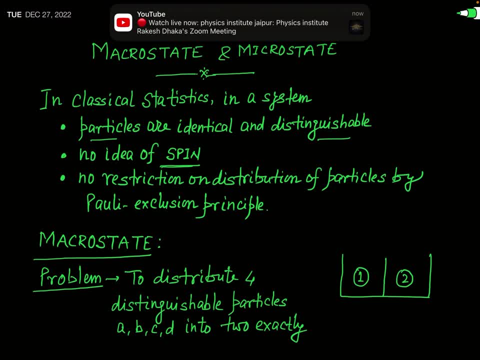 because a spin is associated only with the quantum mechanical system. So here, never think about the spin while you are going to discuss the distribution of particle in different phase cells- okay, or in different compartments, And when this spin is taken under account, then we will start discussing the distribution. 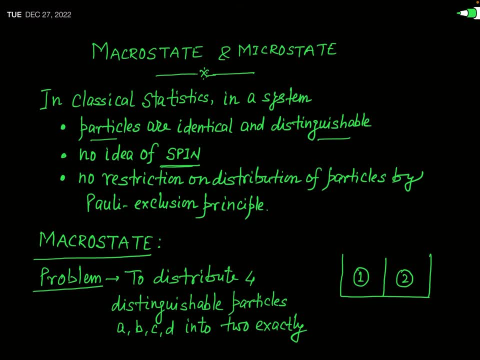 of particle in different phase cells, Then we will study in quantum statistics that there will be two classes of particles known as bosons and fermions. And actually the distribution of fermions in different energy states or in different quantum states is restricted by a very famous principle which is called Pauli's exclusion. 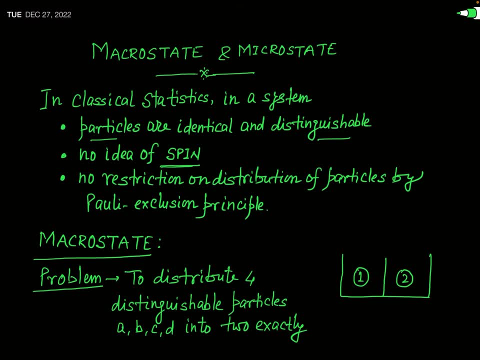 principle, But as a spin is not needed in the discussion of classical system, so we also never think about the Pauli's exclusion principle. So the restriction imposed by the Pauli's exclusion principle on distribution of particles is not applicable in case of the particles of a classical system. okay, 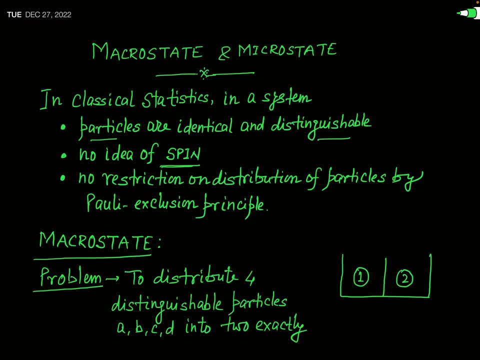 And, as I have told you, that we will explain the concept of macrostate and microstate by taking a very simple example. Actually, when we will take a very simple example and we will talk about these two concepts in terms of that simple example, the concept will be very clear to you. 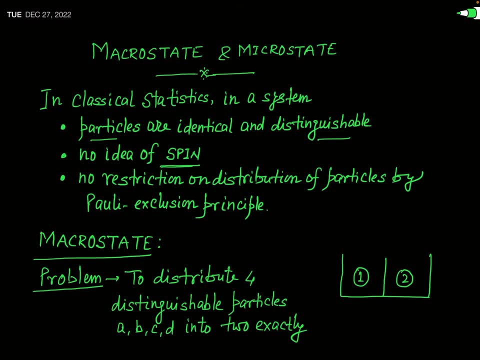 So now, let us start to know. what is this macrostate of a system? okay, Let us consider a problem. there is a system of particles and we have to distribute those particles in the different components. Okay, In the different components, or you can say that in different phase cells of a phase space. 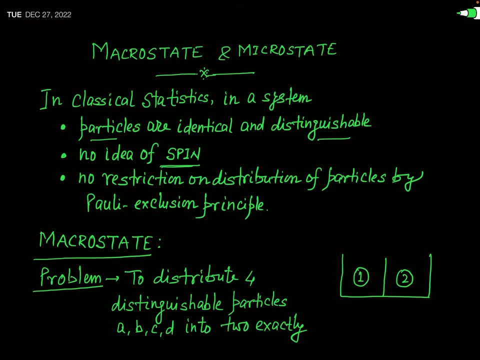 this is our basic problem. So in how many ways we can distribute the given number of particle in different phase cells? this is the basic problem regarding this macrostate And to explain it, as I have told you, we will consider a very simple example. 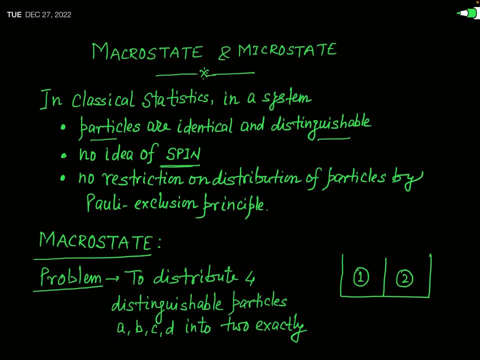 So for illustration, For develop the idea of macrostate, Let us consider there are four distinct particles or four distinguishable particles. okay, So number of particles we consider very small, for simplicity, although in general the number of particles in a classical system is very large, but to develop the idea of macrostate, 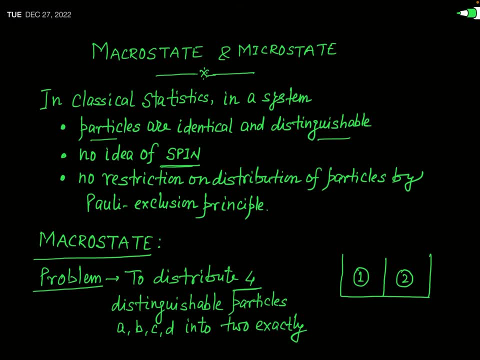 in a convenient manner, In a simple manner. We consider a simple system consisting of four particles and as this system is a classical system, so you can say that, according to the assumption of classical statistics, these particles are distinguishable, and so we can name those particles. 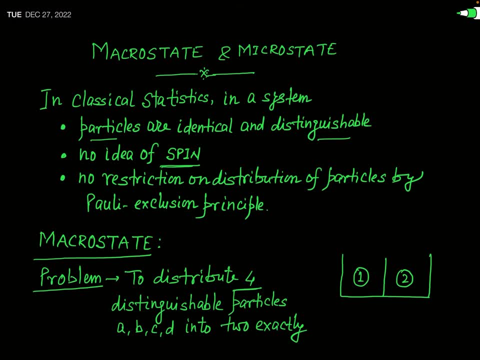 So let us consider the four particles which we have assumed are A, B, C and D, and at any moment you can, you can actually identify that that particular particle is either a or b or c or d. okay, and the number of phase cells or the number of compartments we also consider very small. 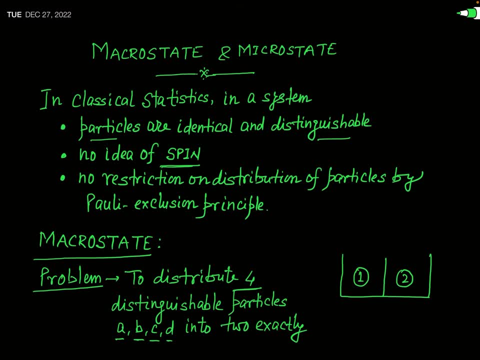 for simplicity, we consider there are two compartments or two phase cells, or in other words, you can suppose that there is an open box, as I have shown in this figure. this is just an open box and this box has actually two compartments, which I have marked here by the number one and two. 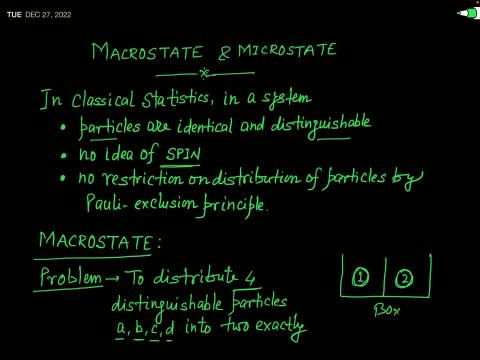 this one and two represents the two compartments, and let us consider that these four particles will be thrown from any place, so that any particle will land, will fall either in the compartment one or in the compartment two. okay, and both of these compartments, or in terms of classical statistics you can say both of these phase cells, are entirely. 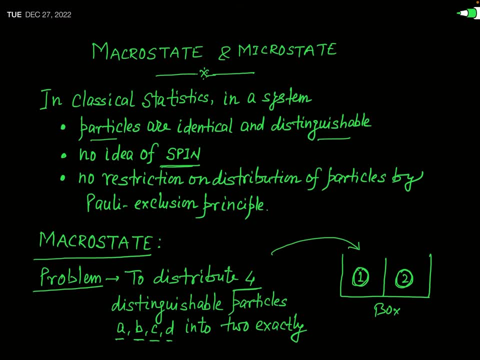 identical, exactly identical, you can say. since both the compartments or phase cells are exactly alike, the particles have the same priory probability of going into either of them. or in other words, you can say that the probability of particles falling into any compartment is one by two, because the particle will fall either in compartment one or in. 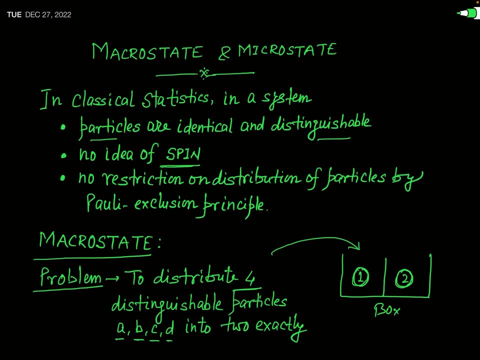 compartment, so two, so that events will be actually the actual number of events taking place will be one, but the two events may take place. so the probability of falling of particles. you can say that the political a divided by co again gives indri VD to Robert troops for quantum. 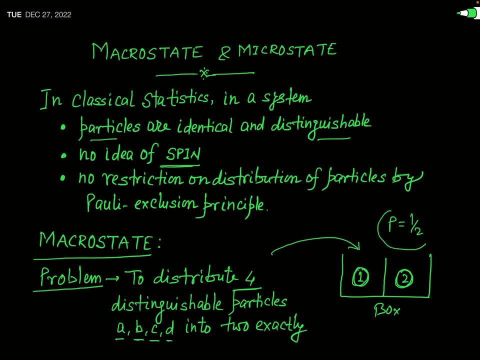 particle in a compartment will be simply equal to 1 by 2. okay, This is actually. this probability is actually known prior to the event, and so this is actually called priory probability. okay, Now the possible number of ways in which these four particles can be distributed in these. 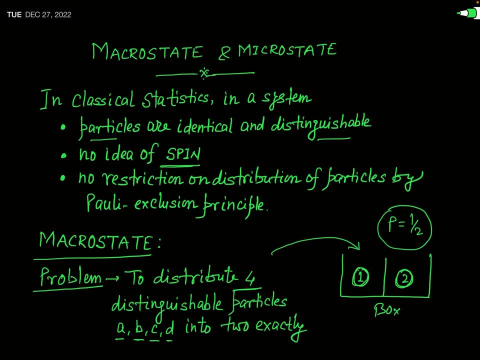 two compartments will be what You can think- that we can consider that in compartment 1 there is no particle and all the four particles are in compartment 2. This may be one of the arrangement. In second arrangement you can consider that one of the particle is in compartment 1 and 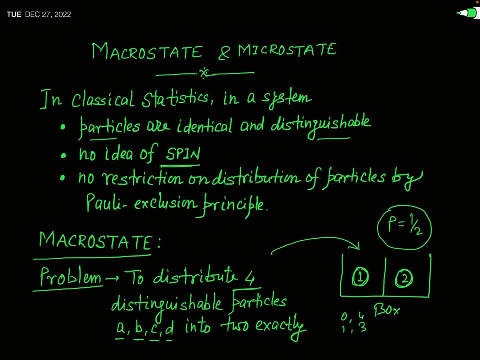 the remaining three is in compartment 2.. So this is the second arrangement. In third arrangement you may take that there are two particles in compartment 1 and the remaining two particles in compartment 2.. So this is the third arrangement. okay, In the similar manner, we also assume that in first compartment there are three particles. 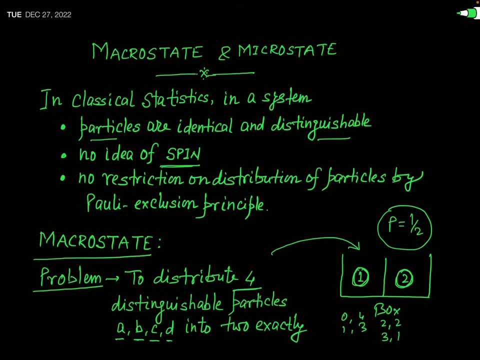 and in the second compartment there is one particle. And in a fifth manner you can consider that all the four particles are in compartment 1. And there is no particle. There is no particle in compartment number 2.. So as a whole you can see that there may be five arrangements of distributing these four. 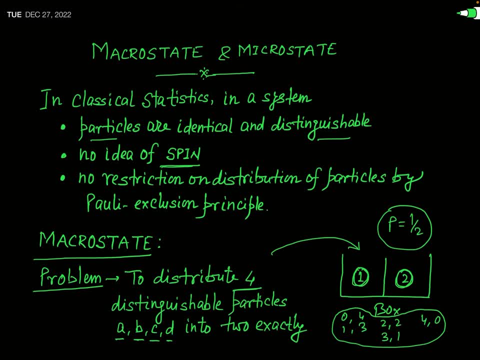 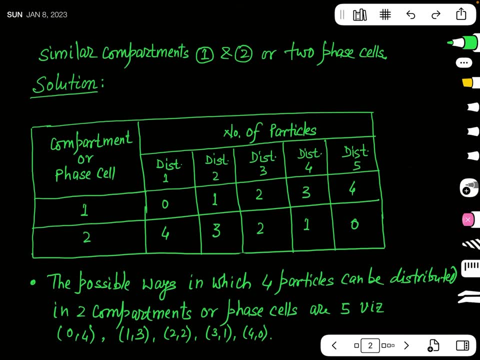 particles into these two compartments or these two phase cells. Actually, I have shown this distribution in tabular form from this table. You can understand this distribution Here. see the table that I have marked Here. you can see the table I have marked here, this one. 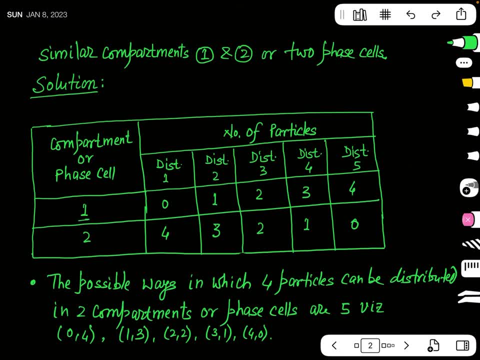 This is actually the number of compartment or the number of phase cell. So this one represents the first phase cell or first compartment, and these two actually represent the second compartment or the second cell. As I have told you just now that if in distribution number one we can consider that there is no 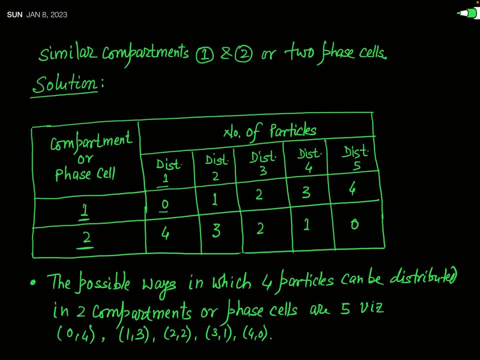 particle in first compartment And all the particles are in the second compartment. So this is one of the arrangement. The first arrangement is 0, 4.. In second distribution you have considered that there is one particle in compartment number one and three in two. 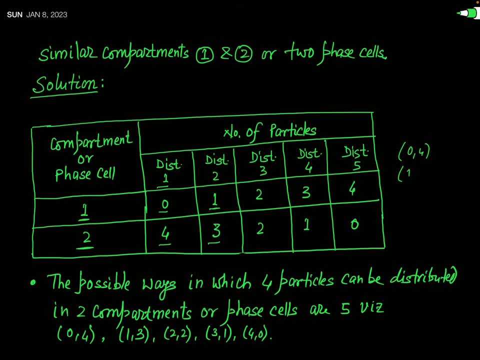 So this is another distinct distribution of particle. This is marked by 1, 3.. And in the similar manner, in the third distribution we consider that there are two particles in compartment one And two particles in compartment two. So this is your third arrangement. 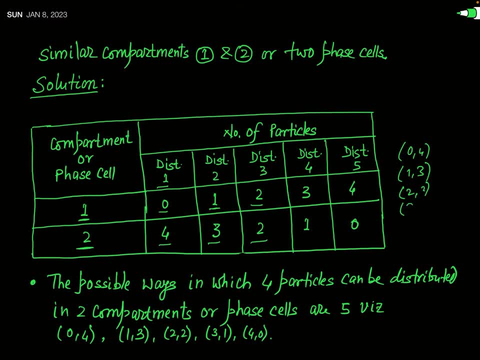 In fourth arrangement we consider that there are 3 particles in the first cell or and the one particle in the second cell. And in the fifth arrangement you consider that all the 4 particles are in compartment number one And there is no particle in compartment 2.. 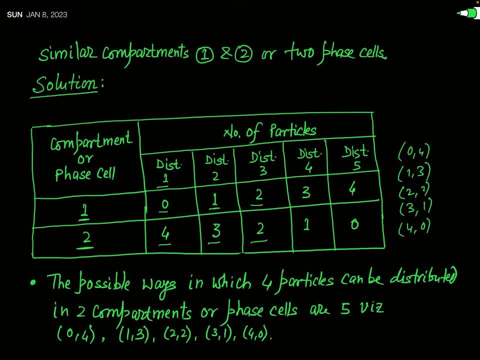 1, 4 and 2 are two cell. So we consider these arrangements. So in as a whole you can say that these are the five distinct arrangement. So if the number of particles is four and the number of compartments will be two in 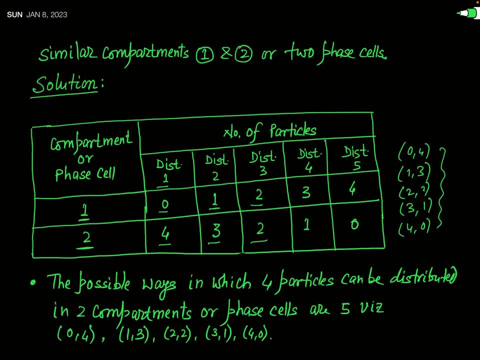 that example, the number of distinct ways of arranging these particles in these two compartments or two phase cells will be simply five. okay, Similarly, this cell wise or the compartment wise distribution of particles is called macrostate. So all these arrangements represent a macrostate. this 0, 4 is one of the macrostate. 1, 3 is another. 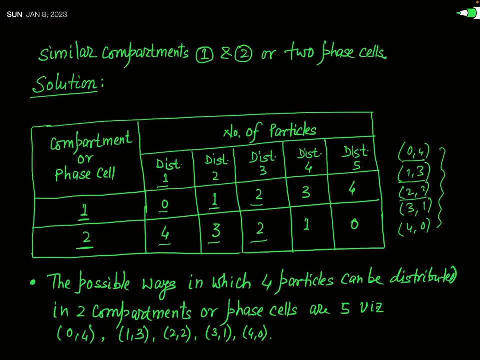 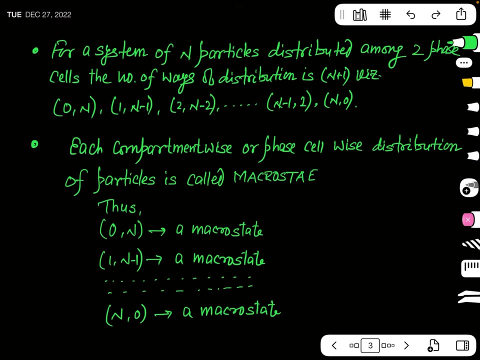 macrostate: 2: 2 is third macrostate, 3, 1 is fourth macrostate and 4: 0 is fifth macrostate. So I have mentioned here, You can see that for a system. so each compartment wise or phase cell wise, distribution of particles. 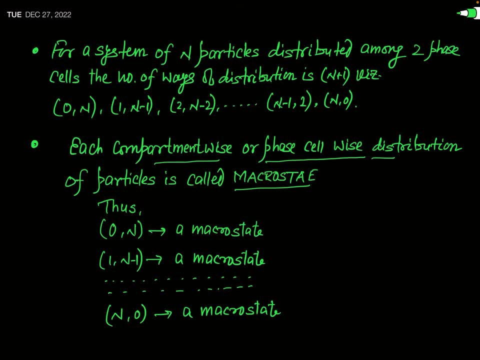 is called macrostate. okay, Now, if we now consider that there are n particles instead of four, we in general consider there are n particles, But even then we consider, Consider that there are there are two phase cells, or the two compartments, and we have to distribute all these n particles which are distinguishable among these two phase. 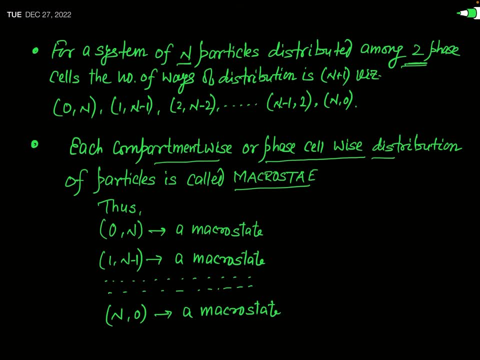 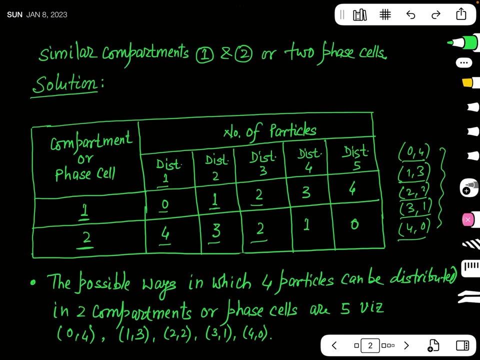 cells or the, these two compartments. Then what will be the number of macrostates? You will see that the number of macrostates will be n plus 1, as in this example, when the total number of Particle was 4. you can see that the total number of macrostates is 5.. 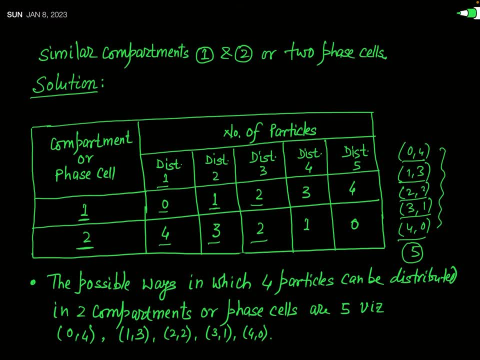 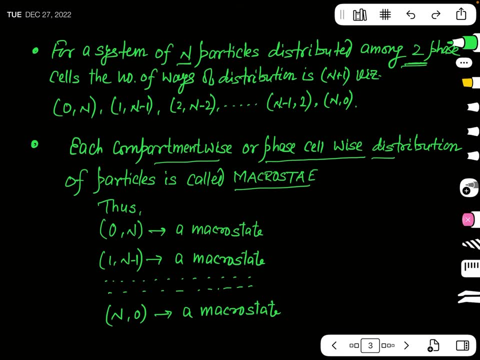 All these represents a macrostate. so the total number of macrostates, when you consider the number of particle 4 and number of compartments 2, then the number of number of arrangements, compartment by arrangements, or you can say the number of macrostate, is 5.. 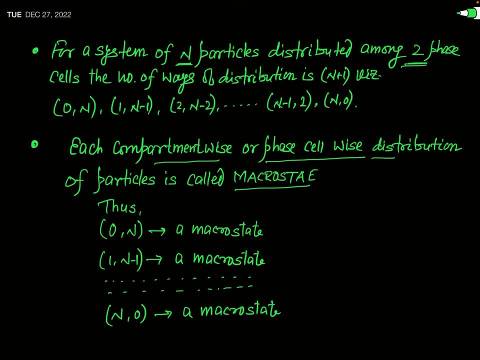 So if there are n particles and all these n particles are to be distributed among the two phase cells or two compartments, then the number of macrostates will be n plus 1. and what will be those macrostates? you can say the first macrostate will be 0, n. it means there is no particle in first compartment. 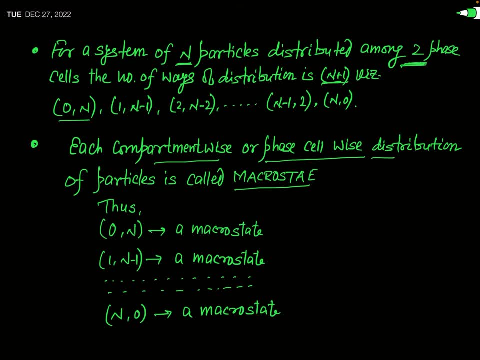 and all n particles are in second compartment, The Another, The second compartment will be 1 and n minus 1. third one will be 2, n minus 2 and similar manner. the nth- sorry, n plus 1th arrangement will be n? 0.. 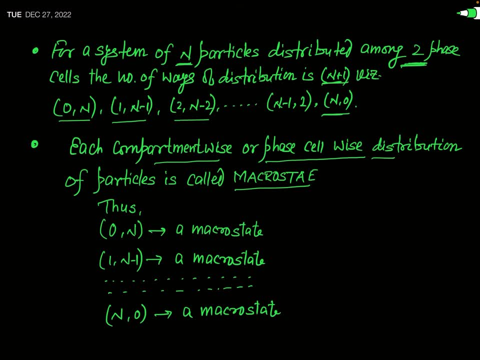 So in this case, if the number of compartments is restricted to 2, but the number of particles in generally n, then the total number of macrostates is n plus 1.. So in this case, if the number of compartments is restricted to 2, but the number of particles 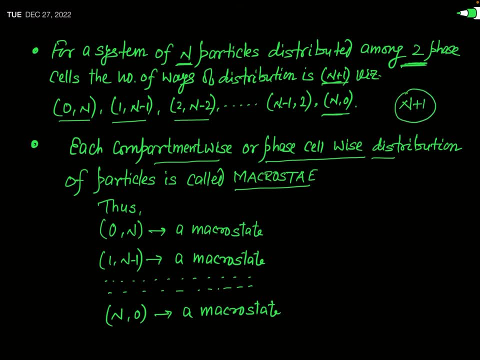 in generally n, then the total number of macrostates is n plus 1. and what are those macrostates? you can see, these are 0, n, 1 minus 1, n minus 1, 2, n minus 2, and so on. ok, So, in fact, as I have told you, that each compartment wise, or phase cell wise, distribution of particles, 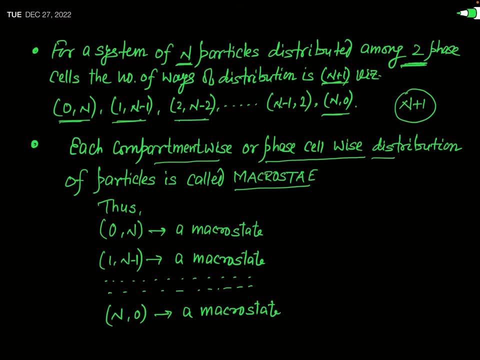 is known as macrostate. ok, So you can say that this 0- n is a macrostate, 1 n minus 1 is another macrostate, And this is actually, you can say, the first macrostate. this is the second macrostate and this will be actually the n plus 1th macrostate. ok, 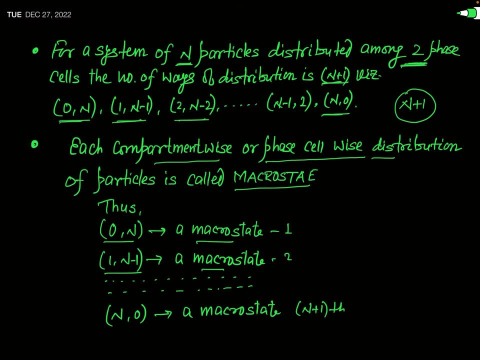 So I hope, from this example, you have definitely understand what is a macrostate. ok, As I have told you, we will clarify the idea by a simple example, And this was a very simple example because we have actually considered the number of compartments 2.. 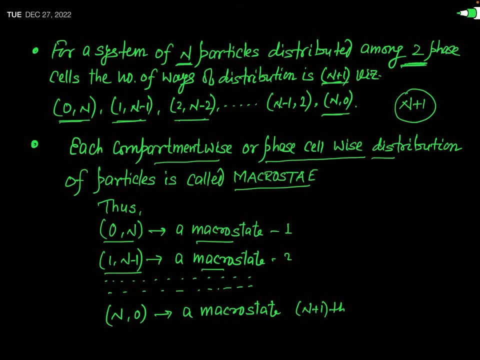 So this was the discussion becomes very simple. But when we will actually solve the actual problem or we will study the classical statistics in the forthcoming lectures, Then there will be not only 2 compartment, there will be a large number of compartments. But generalizing this idea, 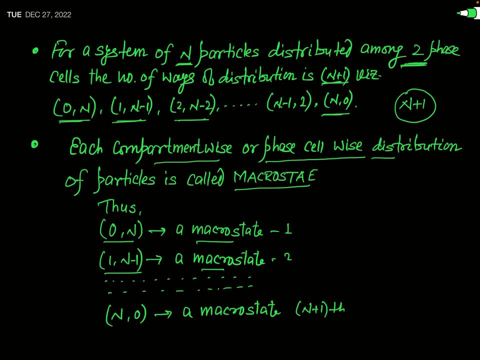 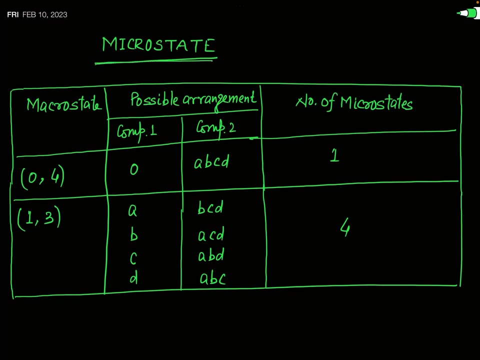 We can find the number of macrostates and what are those macrostates in that examples. ok, So after knowing about the macrostate, now our aim is to clarify the concept of microstate. ok, In fact, in the example which I have just illustrated, you have seen that the particles are distinguishable. 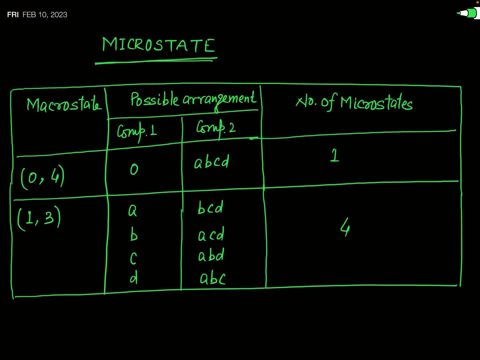 ok, And so that each compartments wide distribution can have a number of different distributions? ok, Because the particles are distinguishable and when you consider the each distinct arrangements for a given macrostate, for a given macrostate there will be distinct arrangement of particles. 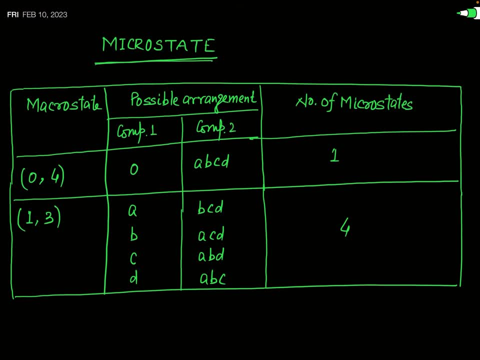 particles are distinguishable, So each distinct arrangement of corresponding to a macro state is called micro state of that macro state. What I am actually telling you, this will be actually clear to you. So let us come see here. We have learnt just now that if there are four distinguishable particles- A, B, C and 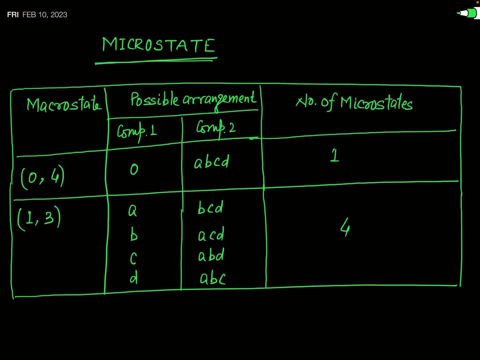 D and we have to distribute them into the two compartments marked by 1 and 2.. Then what was actually the possible number of macro states and what was those macro states? we have already learnt Now we are going to see that how many distinct arrangements is possible. 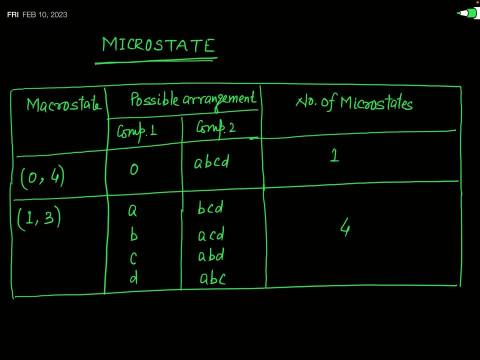 Corresponding to a given macro state, and that number of possible arrangement corresponding to a macro state is called a micro state. Okay, So let us see. See this table, This: all things will be cleared to you by this table. I have shown here that this is your first macro state: 0, 4.. 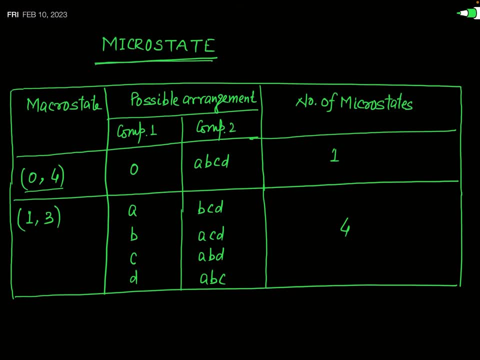 Okay, And when you consider that your macro state is 0, 4.. Okay state is 0, 4, it means in compartment number 1, there is no particle. So I have written here 0.. All the four particles, A, B, C and D, are present in the second compartment, So this is only one. 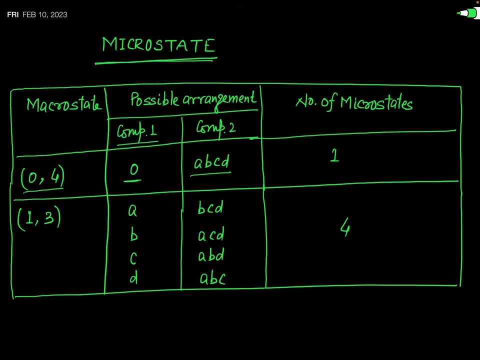 arrangement which will be possible for this macro state: 0, 4.. And as the number of possible distinct arrangement for this macro state is only one, which is 0, and A, B, C, D, So the number of micro states corresponding to this macro state 0, 4 is equal to 1.. 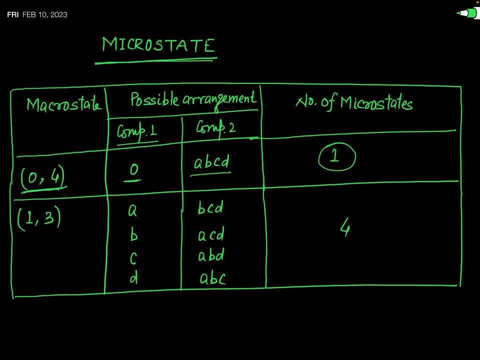 This is the number of micro states, But now let us see the another macro state. Another macro state is what This is: 1, 3.. You have learnt. When you say 1,, 3,, it means there is only 1.. 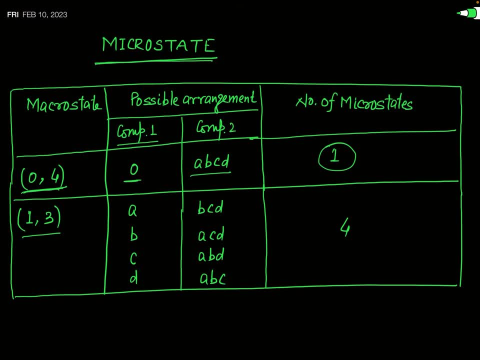 1 particle in compartment 1 and the remaining 3 are in compartment 2.. But as the particles are distinct, so we can consider any 1 in compartment 1 and the remaining in 3.. So if you consider that particle A is in compartment 1, then the remaining 3 particles B, C, D- 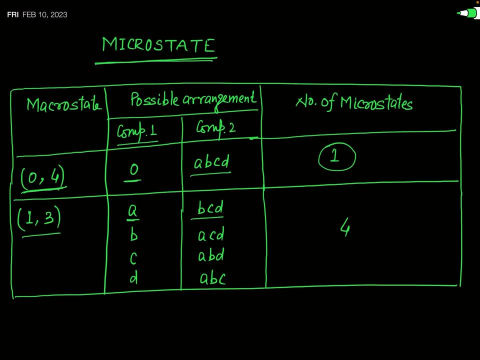 will be in compartment 2, and this is a distinct arrangement. We have considered that A is in compartment 1 and B, C, D are in compartment 2.. But if you consider that particle B is in compartment 1, then the remaining particle- A, C, D- will be in another compartment and 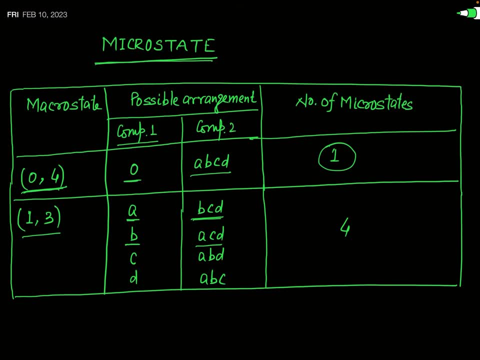 this arrangement is different from the previous arrangement, That is, the arrangement A and B C D and B and A, C D. both are different because particles are distinctly stable And we can also consider that in compartment 1, there is particle C and in compartment 2 is: 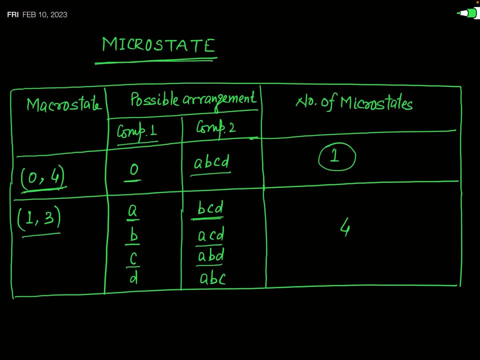 A, B, D and in the fourth manner, you can consider that particle D is in compartment 1 and the remaining particle A, B, C are in compartment 2.. So you can see that, corresponding to this macro state 1 and 3, there are 4 distinct arrangements. All these arrangements- A, B, 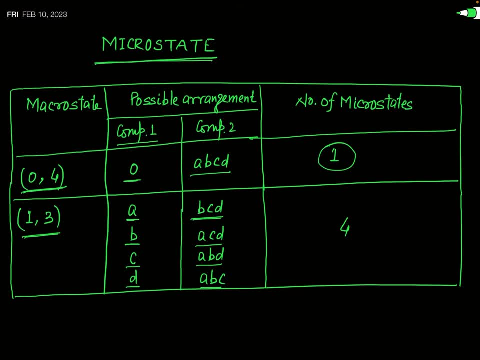 C, D, B, A, C, D, C, A, B, D and D A B C. all these 4 arrangements are different And, as I have told you, that the total number of distinct arrangements corresponding to 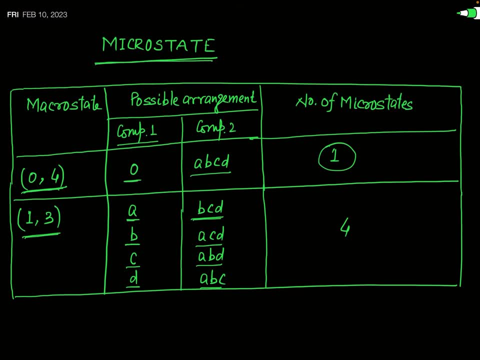 a macro state is the number of micro states. So the number of micro states corresponding to this macro state is what This is: 4.. I think you have understand, And if you have understand, you can see the other examples and you can tell what will. 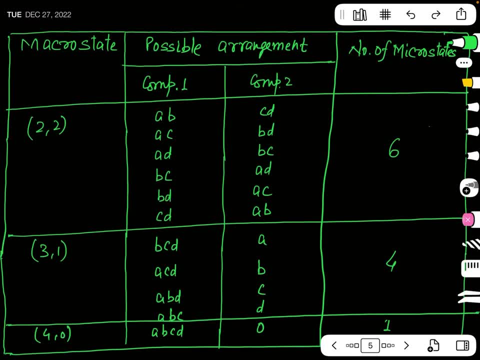 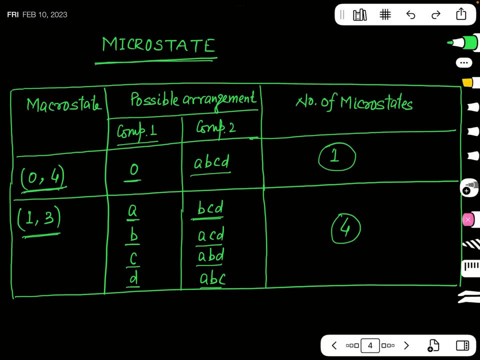 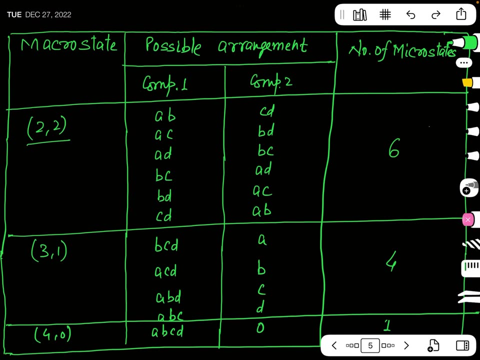 happen. See here, Now we consider the third macro state of that example. This is 2, 2.. When you say 2, 2, what does it mean? It means in first compartment there are 2 particles and in second compartment also there are 2 particles. But what will be that pair of particles? 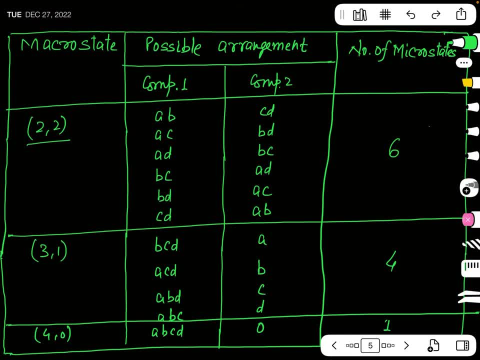 Since the pair, since the particles are distinguishable, so we can take the different pairs. So let us in first set, let us consider that the particles A and B are in compartment 1 and the remaining, C and D, are in compartment 2.. This is a distinct arrangement. Now we consider: 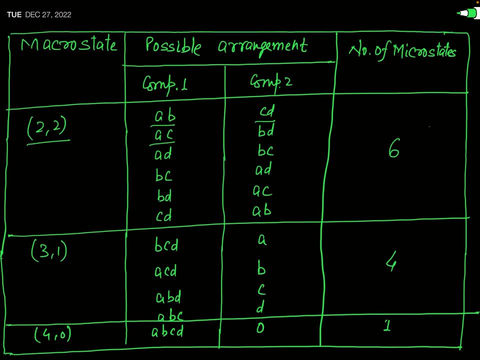 that particle A and C are in 1 and B and D are in compartment 2.. Similarly you can take that particles A and D are in compartment 1 and B and C are in compartment 2. Or at the place of compartment you may also say phase cell, And in similar manner we can. 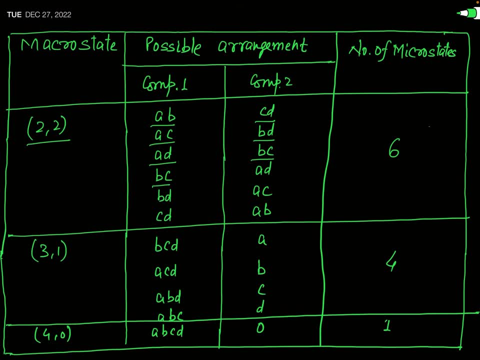 consider that the particles B and C are in compartment 1 and remaining A and D in compartment 2.. And similar manner you can take: B and D are in compartment 1 and A and D are in compartment 2.. And finally, you can take that C and D are in compartment 1 and A and B are in compartment. 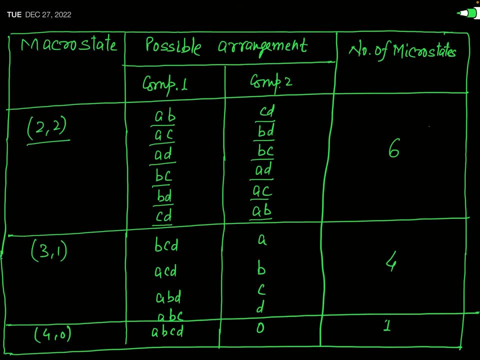 2. Actually, if you will further think that there will be some more arrangement, you will find that there will be not any further arrangement after this. So you can see, all these 6 arrangements are distinct. All these 6 arrangements are different from one another. You cannot say that the arrangement 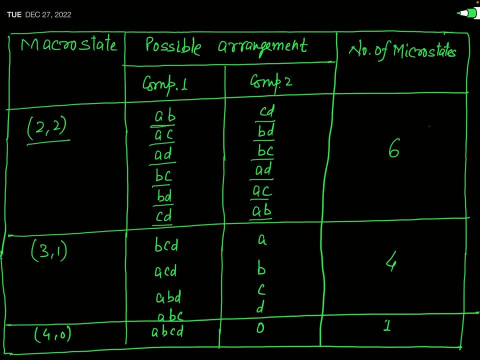 A, B and this C, D, A, B are identical because the particles are distinct. So when in compartment 1, the particles are C and D and in another A and B, and when you consider that in compartment 1, particles are A and B and in compartment 2, these are C and D, So that is, you can say: 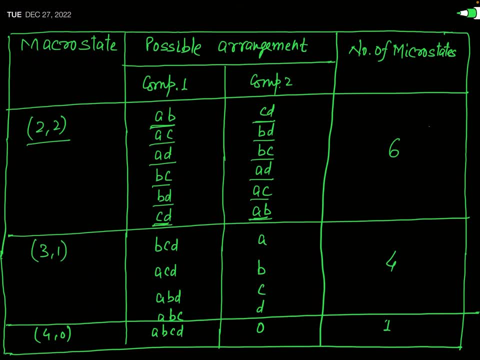 and D. these are different from one another. So you can see corresponding to this macro state, 2, 2. there are 6 distinct arrangement of the particles And as the number of distinct arrangement corresponding to a macro state is called micro state, so for this macro state, 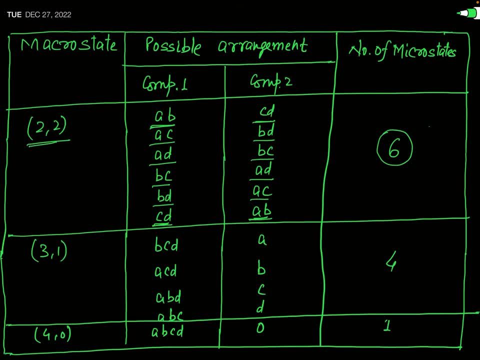 the number of micro states will be what? This will be simply 6.. And in the similar manner, you can see that if we consider the macro state 3, 1, then we will have to place or put three particles in compartment 1 and one in particle 2, one in compartment 2.. 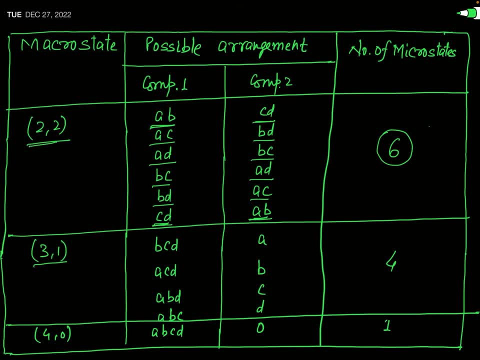 And so let us put the particle A in compartment 2, then the remaining B, C, D will be in 1.. Now place B in compartment 2, then remaining ACD will be in 1. now, if C is in compartment 2, then remaining ABD. 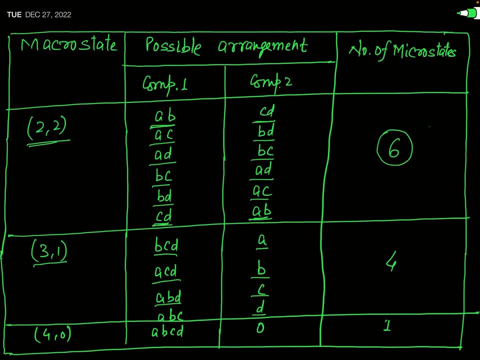 will be in 1, and when D is in compartment 2, the remaining ABC is in 1. so for this macro state again, we find that the number of distinct arrangement of particles among the two compartments are actually 4, so the number of micro states you can say is 4 and in similar 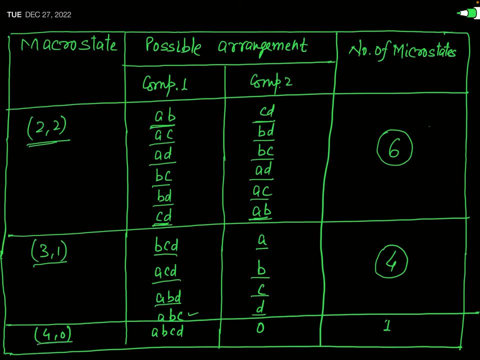 manner for the macro state 4: 0, you will have to put all the 4 particles ABCD in compartment 1 and there will be no particle in compartment 2, and so, corresponding to this macro state, there will be only one arrangement and so the number of micro states. 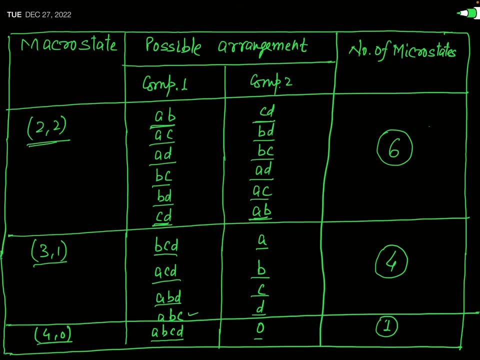 for this macro state is 1. okay, so I think you have understand how this micro state is different from the macro state. in nutshell, you can say that when you talk about macro state, that is simply the number of arrangement of particles in compartments or in phase cells. 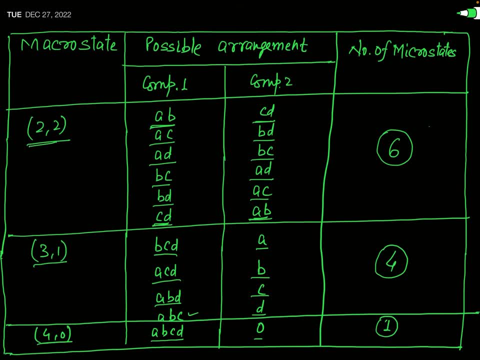 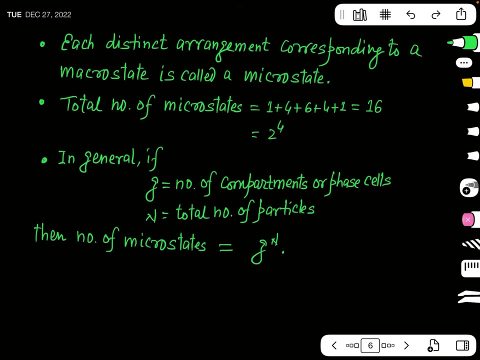 but when we take into account what will be the distinct arrangement of particles among these phase cells that represent the micro states. now, in this condition, what is the total number of micro states? you can easily see the total number of micro states from this example. you can see this will be 1 plus 4 plus 6 plus 4 plus 1, that is 16, and this 16 can be written as 2. 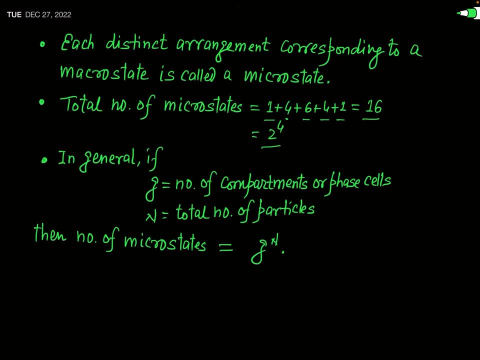 to the power 4. why I have written 2 to the power 4. you can note it as 2 too. that is 1 plus 4 plus 6, P plus 1 or plus 16. this 16 can be written as 2 to the power 4. Why I have rBM: 2 to the power 4. you can note this as 2.. 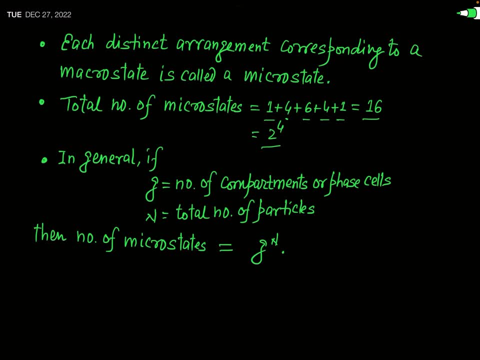 understand. actually this is a general result if you consider that here actually this 2 represents the number of compartments, or the phase cells, and this index 4 represents the number of particles. ok, So in general, if you consider that there are g number of compartments, g represents the 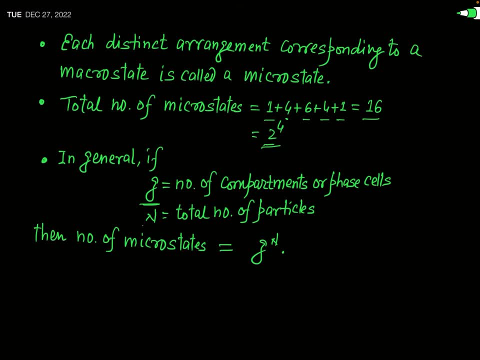 number of compartments or number of phase cells, and n represents the total number of distinguishable particles, then for that system the total number of microstates will be g to the power n, g to the power n. For example, if you consider that there are 3 phase cells or 3 compartments, and n is equal, 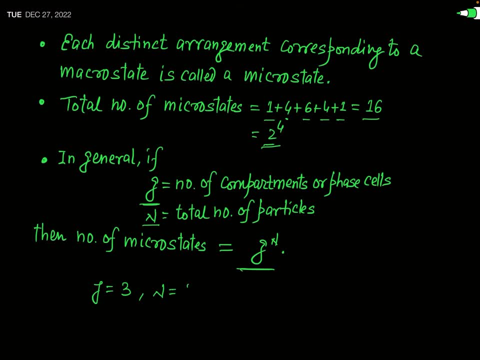 to, let us say, 3.. n is equal to also 3, then what will be the total number of microstates? that will be 3 to the power, 3 and that will be 27. ok, So in this way, remember this result, that if g represents the number of compartments, or 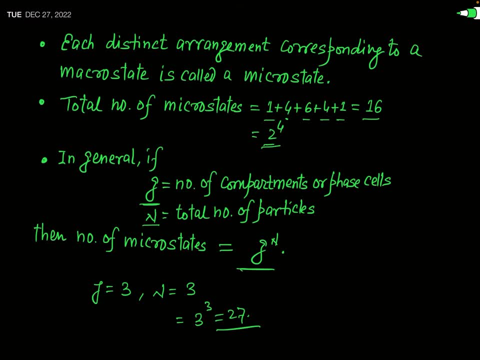 number of phase cells and n is the total number of particles which are distinguishable. then the total number of microstates will be equal to g to the power n. total number means the sum of the micro number of microstates corresponding to the different macrostates. ok, different macrostates. 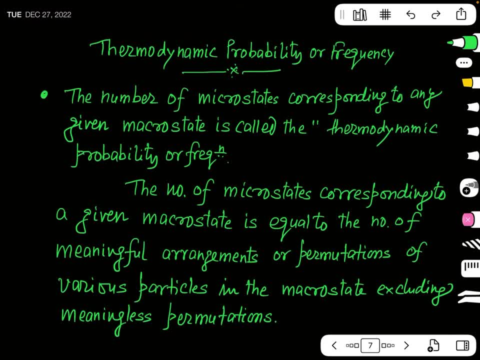 So I think, from this simple explanation, by taking simple example, I definitely the idea of macrostate and microstate. I have been clear to you. ok, Now we will see another concept, which is actually regarding the thermodynamic probability, or you may also say it thermodynamic frequency. ok, thermodynamic probability or thermodynamic. 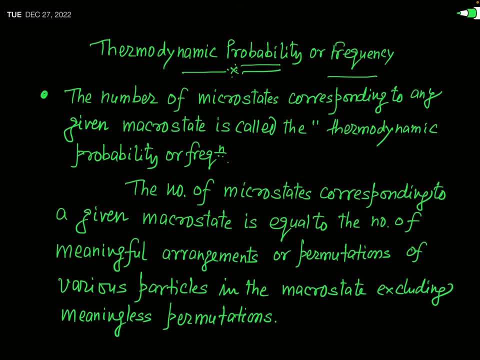 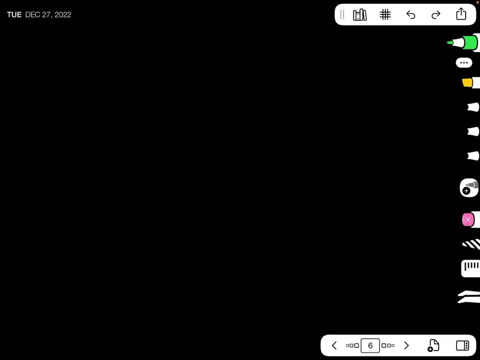 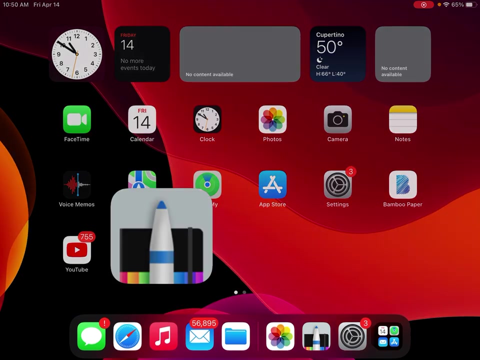 frequency. Actually, this thermodynamic probability is what? this is nothing. this is simply the Number of microstates corresponding to any given macrostate. as you have seen in this example, that corresponding to this macrostate, let us say 2, 2. sorry, the phase has been turned. 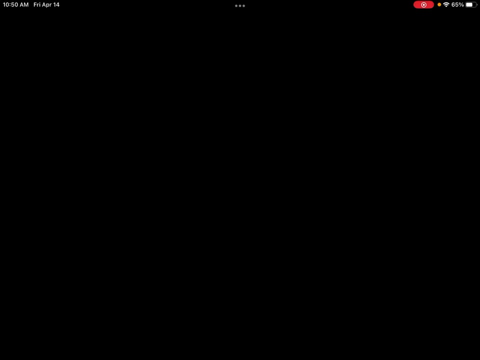 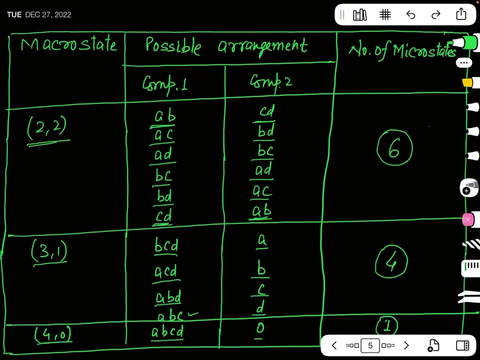 but this will be just ok. So see here: The macrostate which I have considered Is 2, 2.. And you can see corresponding to this macrostate: 2, 2. the number of microstate is what this is 6.. 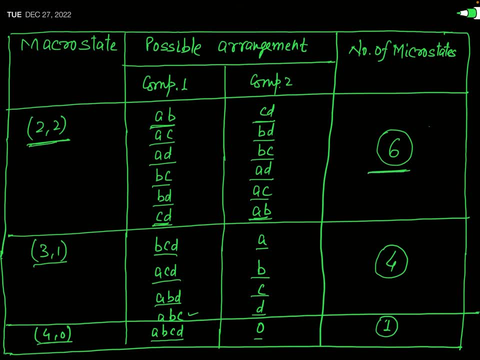 In simple manner, this number of microstates, which is 6, for the macrostate, which is 2, 2, this 6 is called actually the thermodynamic probability or thermodynamic frequency of this macrostate. So if I will ask you that, what is this for this poor is the number of microstates corresponding. 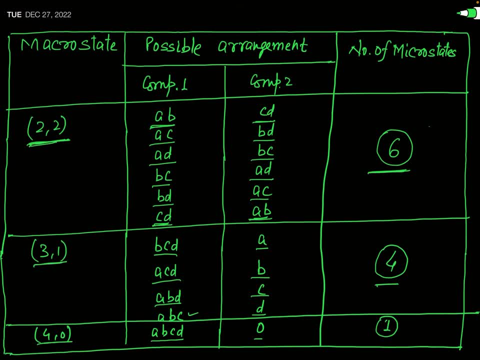 to the macrostate 31. so if I Will ask you that, what is the thermodynamic probability of the macrostate 31, what is the thermodynamic probability of Macrostate 31.. What frequency of macrostate 31? your answer will be what? your answer will be 4 because thermodynamic. 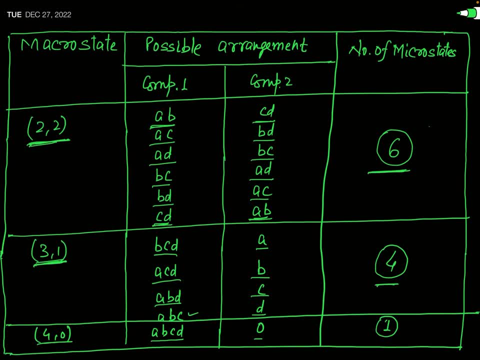 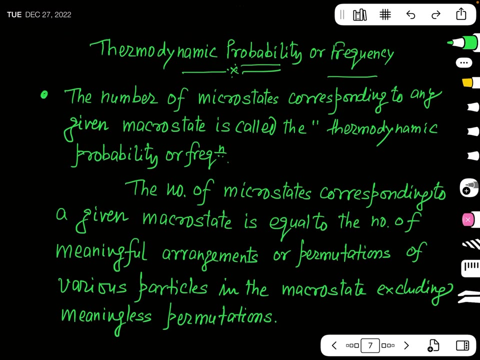 probabilities simply represents the number of microstates corresponding to a given macrostate. okay, so there is no difference between the number of microstates and the number and the thermodynamic probability or frequency for a given macrostate? okay, so I have mentioned it here. you can see that the number of microstates corresponding to any given macrostate is called. 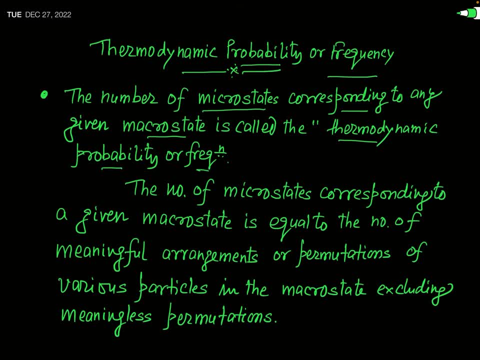 thermodynamic probability or frequency. okay, now what will be? it will be actually the thermodynamic probability or frequency. you can see, actually, when you say that this is just equal to number of microstates corresponding to a given macrostate, actually the microstates represents the meaningful arrangements, market meaningful arrangements. 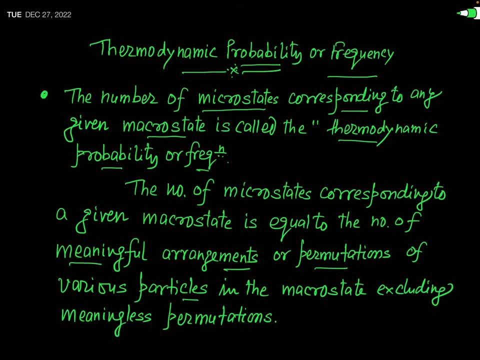 or meaningful permutations of various particles in the macrostate, excluding the meaningless permutations. there may be meaningless permutations when you, for example, if you consider the fact that there is a particle and that will be replaced and another identical particle will acquire that position there, actually then there will be no creation of new estate. so if you count, 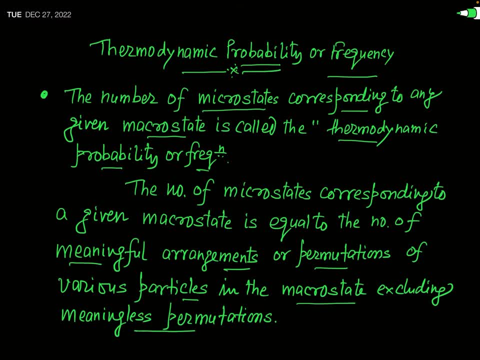 the number of estates or number of microstates in that condition, taking that permutation too, that will be wrong. that is called meaningless permutation. so in the meaningless permutation, the number of meaningful permutations or the number of meaningful, number of meaningful ways of distribution of particles, that is actually called the thermodynamic. 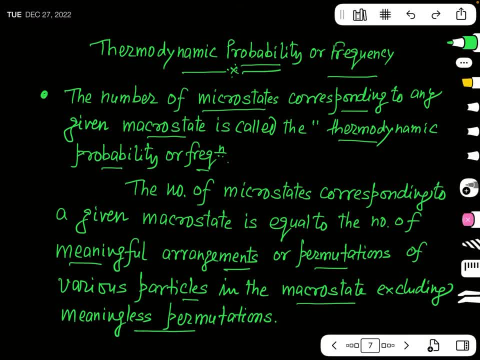 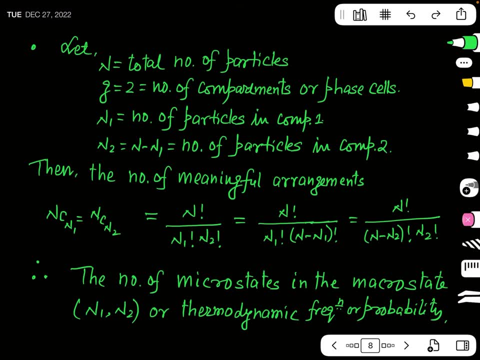 probability. okay, now we will again formulate this idea by a simple example. for this, let us consider: the total number of particles in our classical system is equal to n, but here again, to clarify the concept in a simple manner, we restrict ourselves to the number, to for the number of phase cells or number. 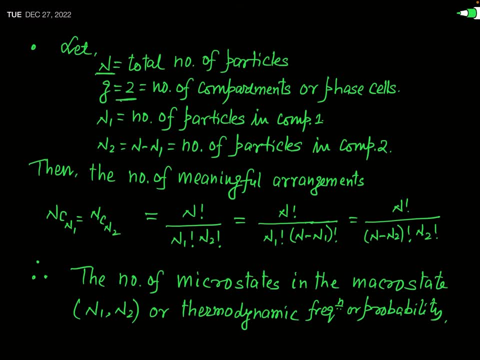 of compartments. at 2 I have considered that there is only two phase cells or only two compartments. for simplicity, okay, but the number of particles in the system is n. okay, it means say these n particles are to be distributed among the two cells. this is cell number, let us say one and this is two. so if you consider that n1 is the number of particle in 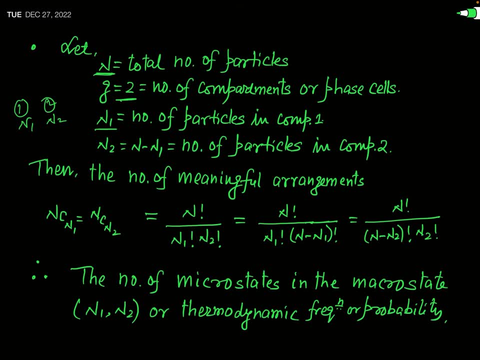 first cell and n2 is the number of particle in second cell. when you say n2, that means the remaining number of particles, and remaining number will be what that will be: n minus n1, so that n? 2 will be simply equal to n minus n1. okay, so you can say that among these two 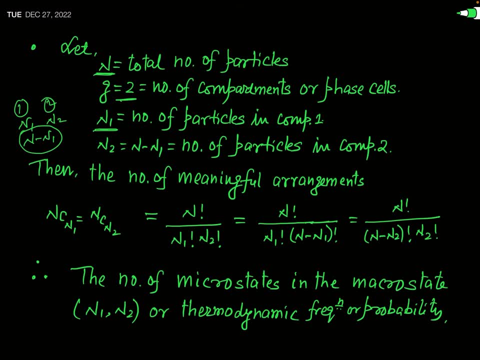 cells, n1 is the number of particles in first cell and n2, which is equal to n minus n1, that is the number of particles in second phase cell or second compartment. in fact, in that condition you have definitely studied the permutation and combination in your course on algebra and definitely you. 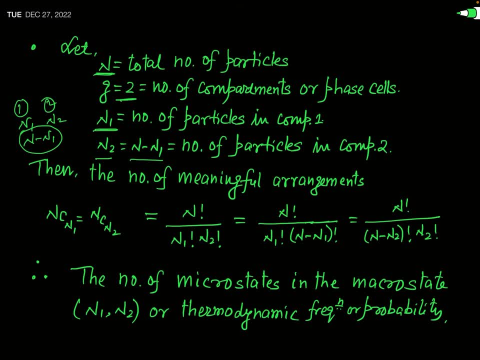 have an idea of it that the number of meaningful arrangement in this condition will be what. that will be simply nCn1, or you can also say nCn2. value of nCn1 and nCn2 are same. you have definitely an idea of this. and when you say nC1, 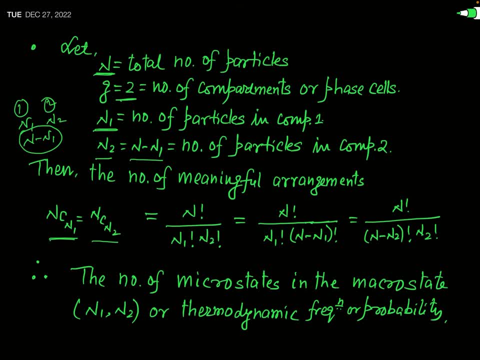 nCn1. that means what that is: n factorial divided by n1 factorial times n2 factorial, and in a state of this n2 factorial, you can write n minus n1 factorial. or in a state of this this n1 factorial, you can write n minus n2 factorial and n2 factorial. okay so? 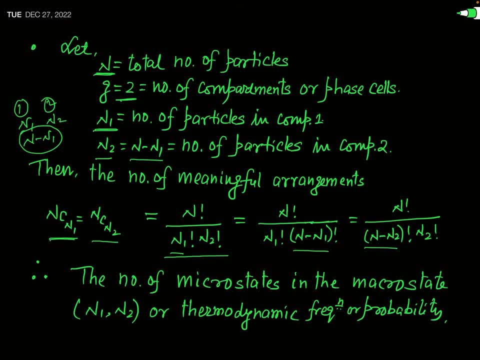 the number of meaningful arrangement of n particles among the two phase cells or among the bit among the two compartments, will be simply equal to nCn1 or nCn2, and which is equal to this much, ok, but as I have told you that the number of 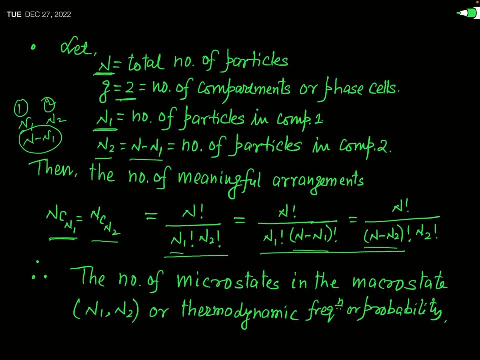 meaningful arrangement of particles among the phase cells represents actually the number of microstates, or you can say the thermodynamic probability. so the thermodynamic probability in this case will be simply equal to nCn1 or nCn2. so I have mentioned it here. you can see that the thermodynamic 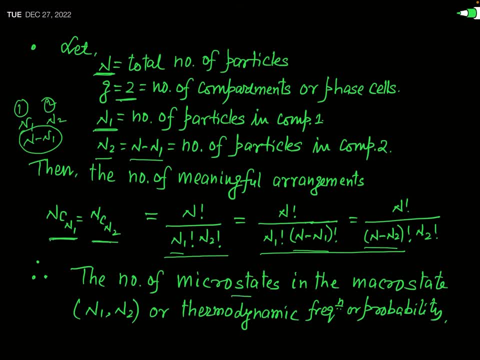 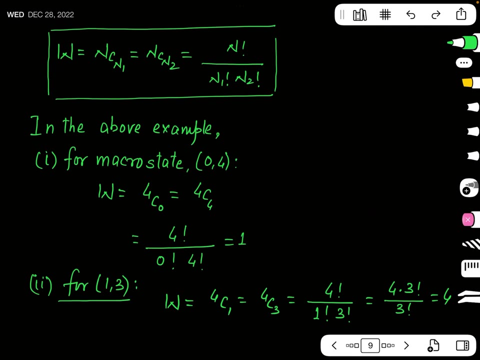 arrive. stability in this case will be simply equal toNn or Nn2, so I the number of microstates in the macrostates N1, N2, or the thermodynamic frequency or probability. this will be what This is actually equal to if we denote this probability by the symbol W. 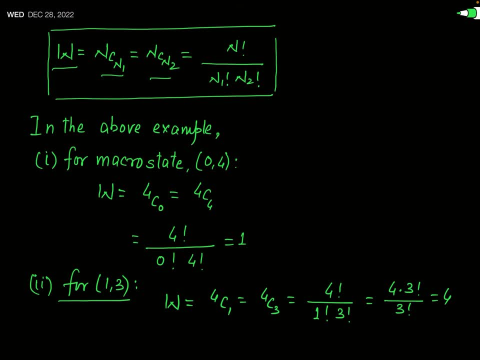 that W is equal to NcN1 or NcN2 and that will be equal to N factorial divided by N1 factorial times N2 factorial. You can check this formula because we have already calculated the number of microstates corresponding to a given macrostate. 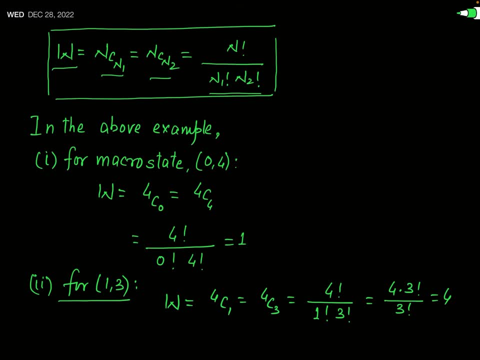 In our previous example you can see. So, as you have considered four particles distributed among the two phase cells, or two compartments, the first macrostate was 0,4.. So now let us find the number of microstates, Or the thermodynamic probability for this macrostate, from this formula. 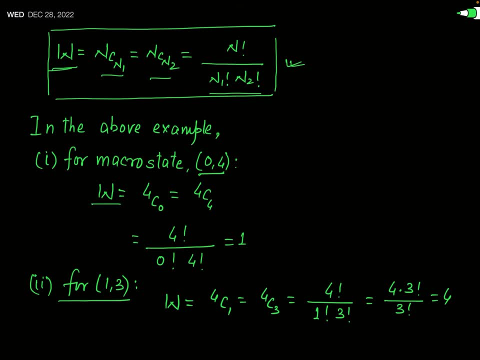 Let us try to find. You know that the thermodynamic probability, W, or the number of microstates will be what? Because formula is NcN1.. Here N means 4 and N1 is 0. So this is 4C0 or NcN2.. 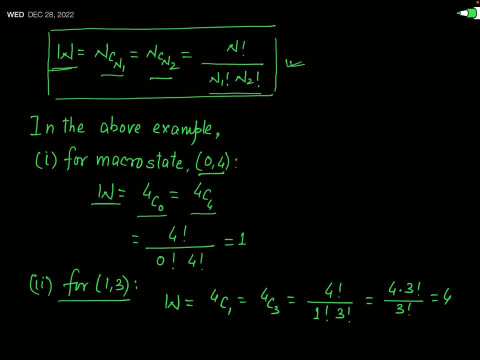 N2 is 4.. So this is 4C4.. And what will be this? This will be 4 factorial divided by 0 factorial times 4 factorial. You know, 0 factorial is what? This is equal to 1.. 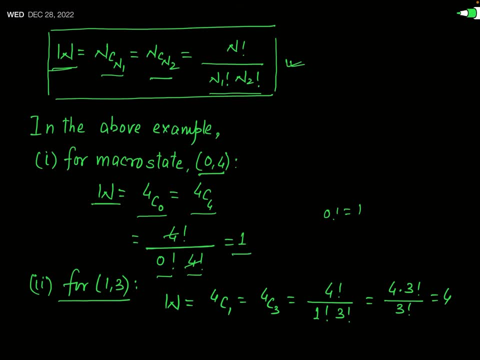 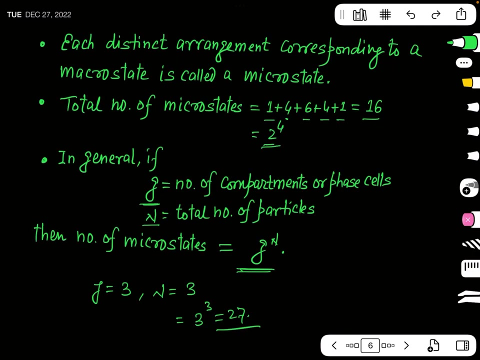 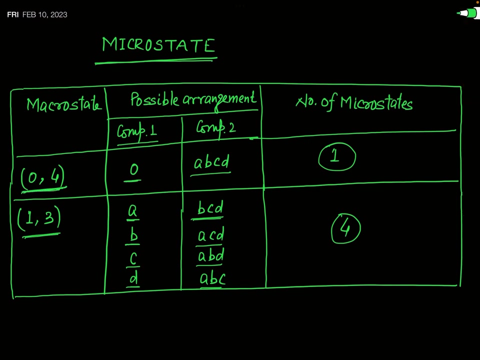 So this 4 factorial and 4 factorial will cancel and this comes out 1.. So what is the number of microstates or the thermodynamic probability corresponding to the macrostate 0,4?? You can see. So this is 1 and the same thing you have seen earlier in this example in tabular form. I have already mentioned. you can see this: for this macrostate 0,4, the number of microstate is 1,. okay. 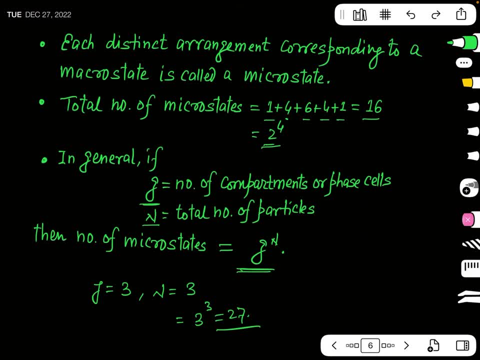 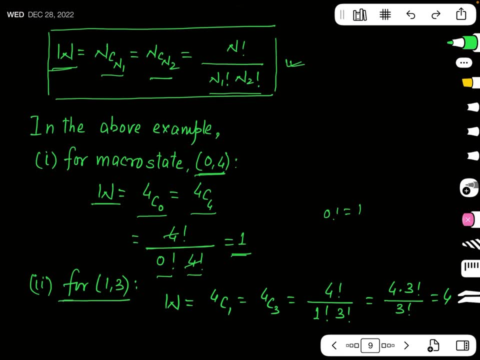 So that formula is correct, you can check. okay, Now let us take the another example. This is the macrostate 1,3.. Okay, so here N1 is equal to 1 and N2 is equal to 3.. 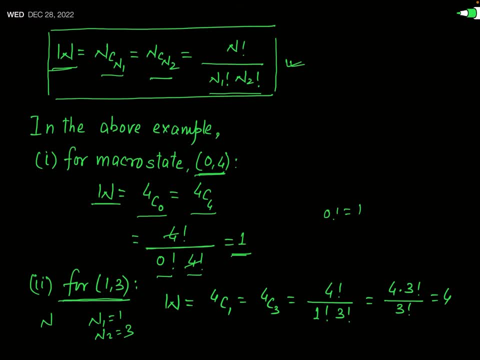 So you can write it. and the total number of particles N is equal to 4.. So you can write this: thermodynamic probability will be equal to 4C1 or 4C3.. This is NcN1 or NcN2.. 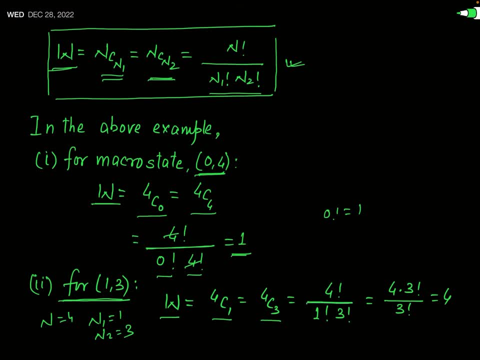 And that will be simply equal to 4 factorial divided by 0. So NcN2 is equal to 4 factorial divided by 1 factorial times 3 factorial. Now 4 factorial. you can write this is equal to 4 times 3 factorial and 1 factorial, you know, is equal to 1.. 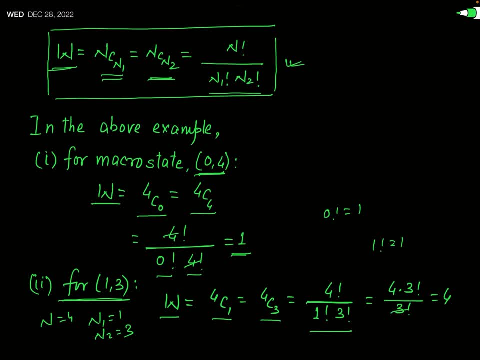 So I have not written it here as: and 3 factorial. So this 3 factorial and 3 factorial will cancel and your result is 4,. okay, And you have seen earlier that for this macrostate, the number of macrostate is 4.. 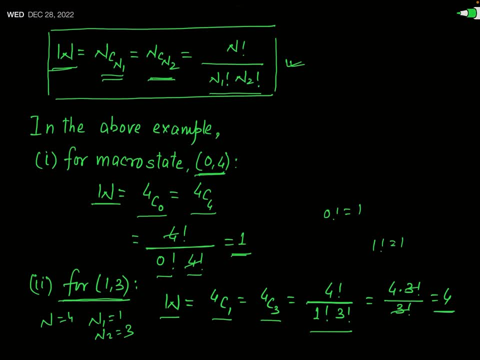 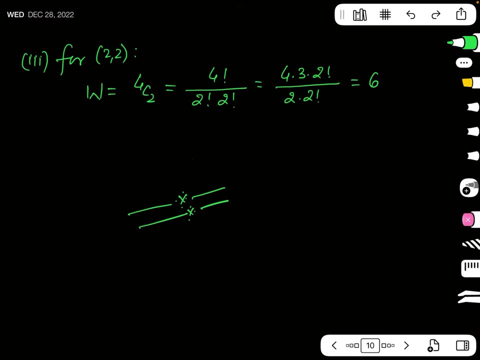 So the formula is checked, okay. And in the similar manner, now try to find the number of microstates or thermodynamic probability for this macrostate, 2,2.. Here, actually, N1 is equal to 2 and N2 is also equal to 2, okay. 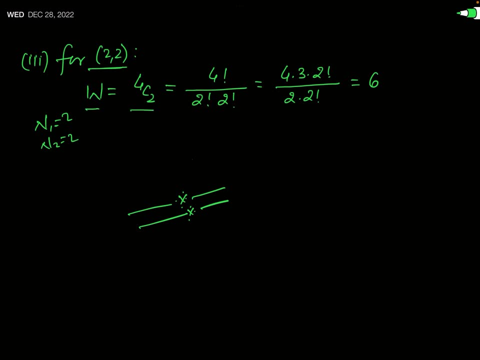 So from that formula W is equal to 4C2 and that will be 4 factorial. So this is 2 factorial over 2 factorial times 2 factorial, Now 4 factorial. you may write 4 into 3, into 2 factorial. 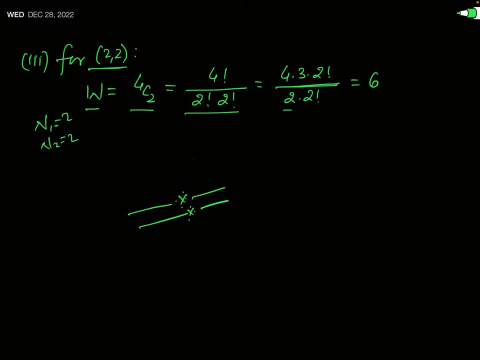 And 2 factorial is simply equal to 2 into 1, that is 2.. And this is 2 factorial. This 2 factorial and 2 factorial will cancel. This is 2 times 2.. So 2 times 3 is equal to 6.. 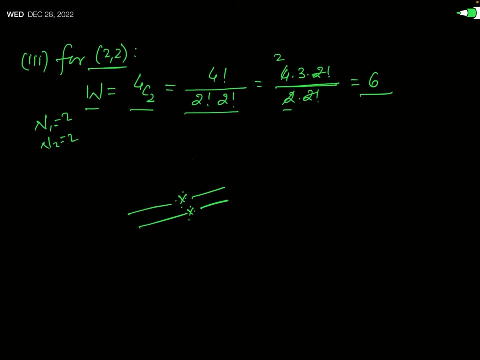 And that's why you can say that the thermodynamic probability, or the number of microstates corresponding to this macrostate, 2,2, is equal to what This is 6,. okay, So from these examples, definitely you have a concrete idea of the macrostate and microstate. 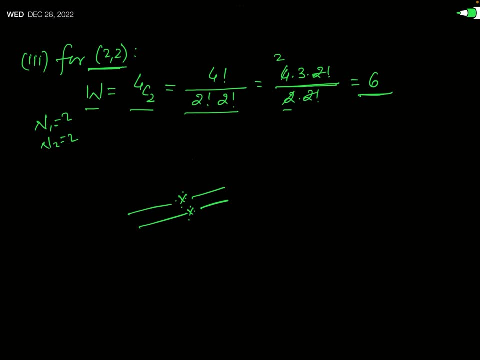 It is just a deep belief in you. Have you understand or not? Actually, when you follow a textbook, the idea of macrostate and microstates are written in vague and so the students, most of the students, get confused. But I think from my this video, which is very simple, to understand the concept of microstate and macrostate. 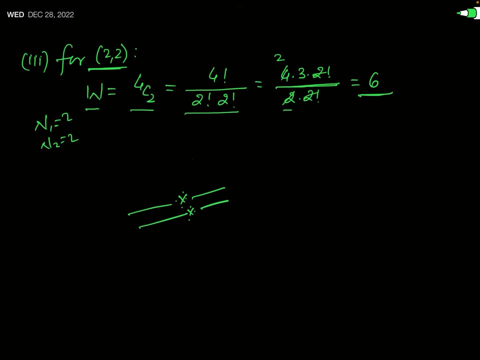 this concept of macrostate and microstate will be definitely very clear to you and the manner you will find very convenient to understand this idea. And so watch the video seriously and write your comment in comment box, And if you have any problem or any doubt, you may write in comment box. 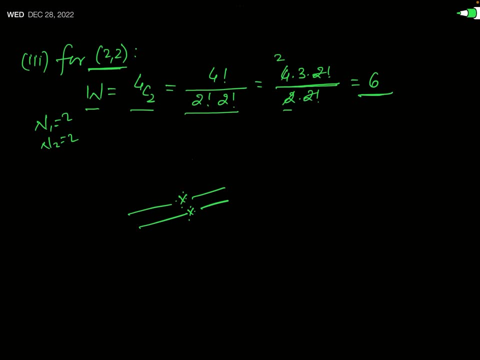 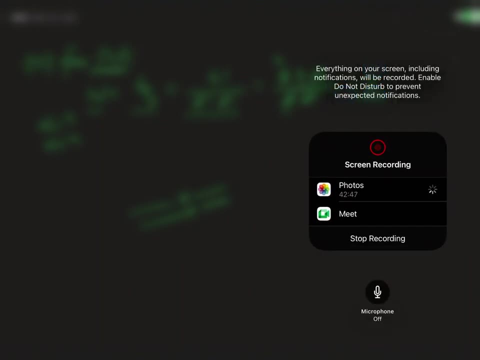 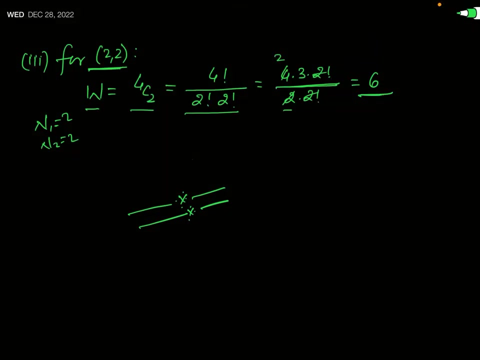 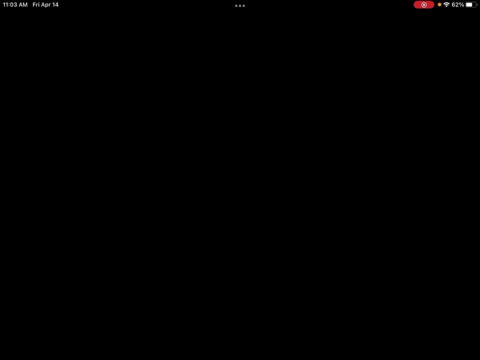 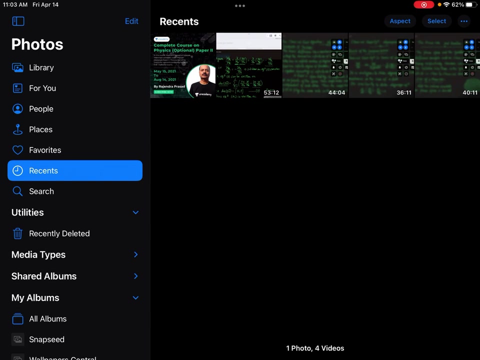 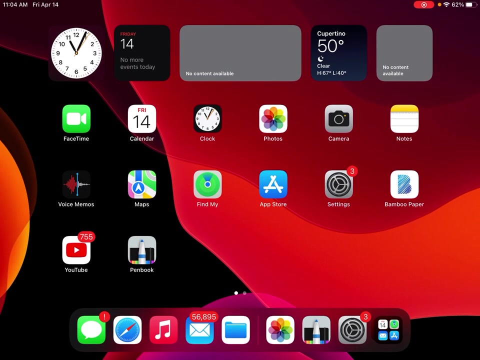 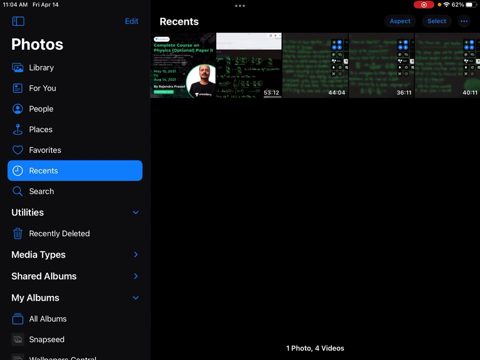 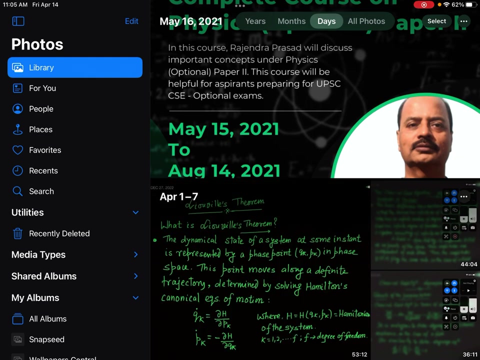 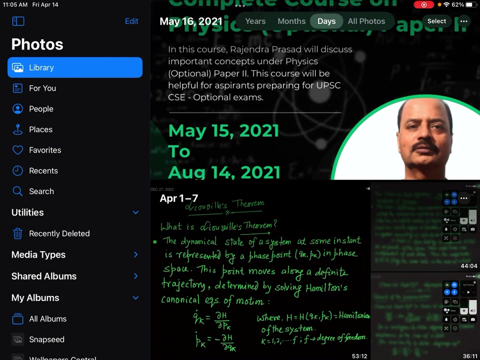 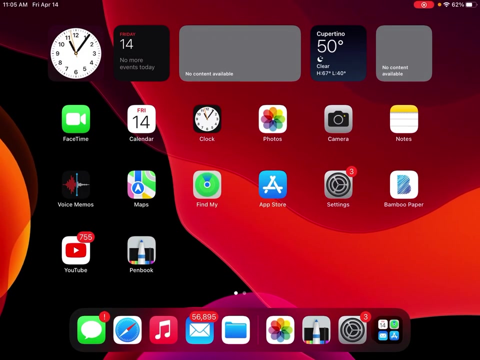